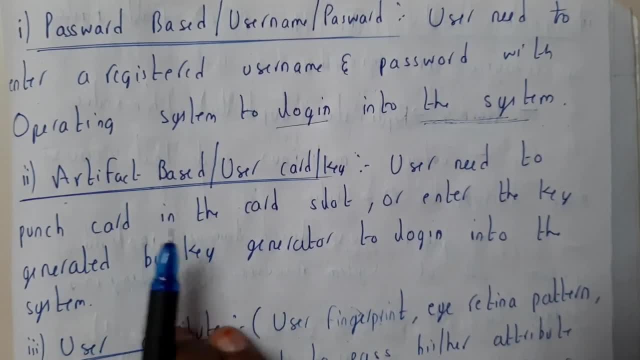 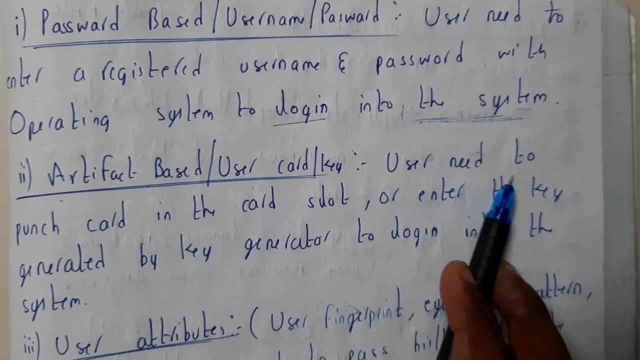 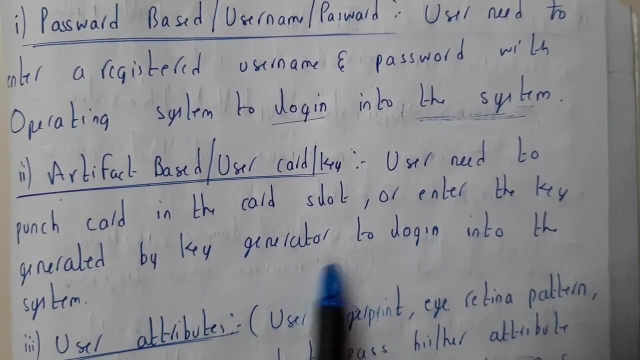 method: Fine, Okay. And artificial based systems or artifact based systems or using cards or keys. User need to punch card in the card slot or enter the key to generate, generated by the key generator to login into the systems. Basically, these are used in some: 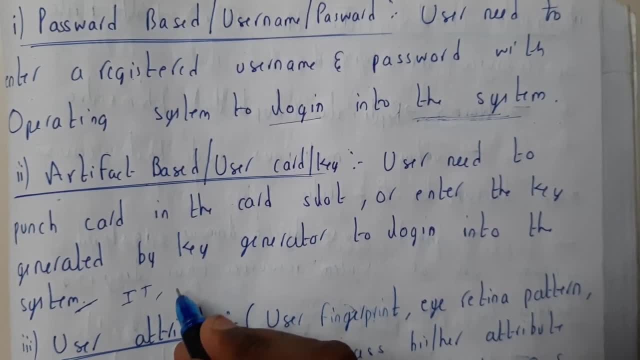 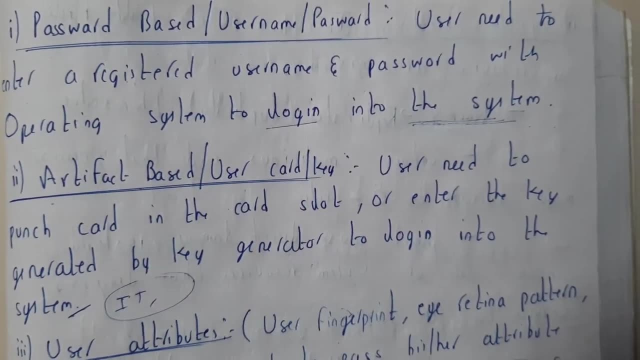 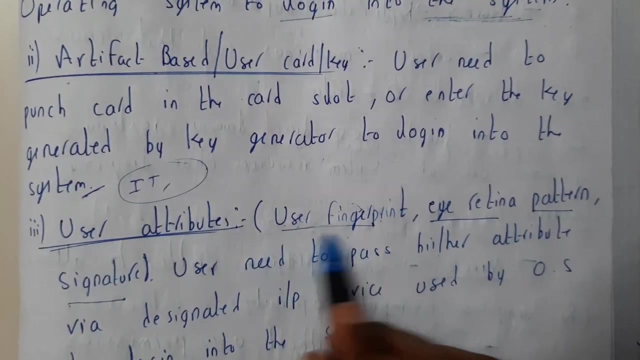 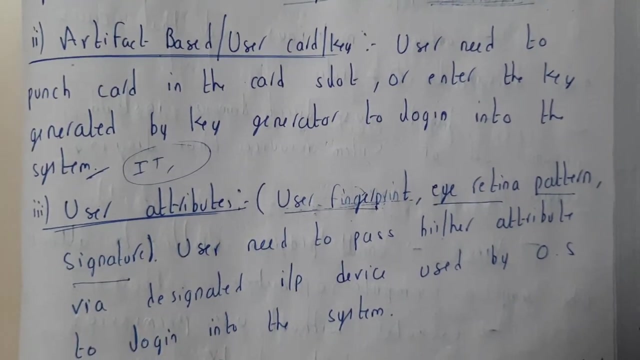 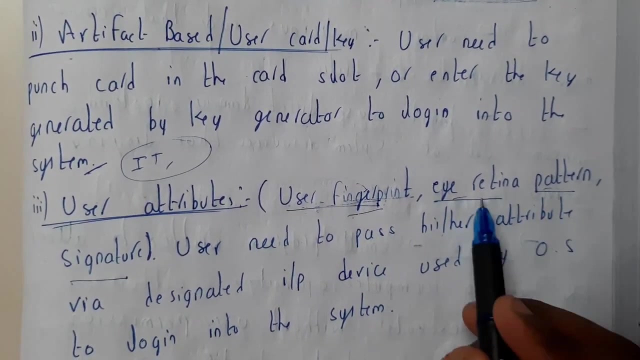 IT companies and mainly in space stations like NASA and few other places. So these are the existing ones that we are going to use in future. I hope basic information starts teaching you so well, So we will be checking out in this video how to do. these Here. the purl sense is coming funny, So I forget to say that it already came. So I, with a number of away случай g buttress is very huge and very cheap this size. So what I am showing today is. what I am showing today is we are going to see now what is the common product of Dannemberg. Artifact and artificial cards And what are the capabilities of come here. the protection is really hi guys. okay, so by user attributes, by using fingerprints. I retina patterns and signatures. So basically these fingerprints will be used in the bank systems. bank bank employees will be using the thumbprints to log into. 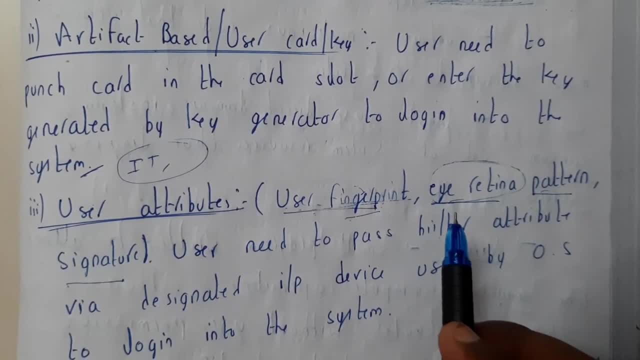 their systems. okay. so basically, I hope everyone knows this about, because we are using these things in a mobile fingerprint. Basically it should scan iRetina, but it will not scan iRetina. It will just scan the outer structure of your face and, according to it, it will be unlocked. 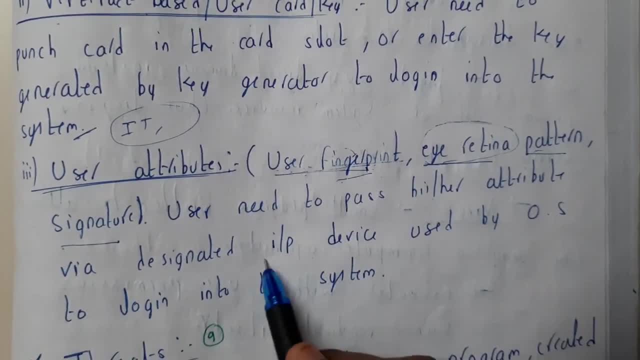 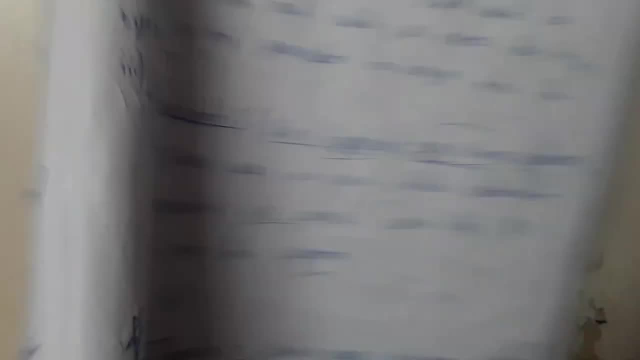 So user need to pass his or her attributes via a designed input device- yes, used by an OS to log in into the system. So I hope everyone got a small idea on authentication. So in the next tutorial we will be going through the next concept. that is nothing but threads. 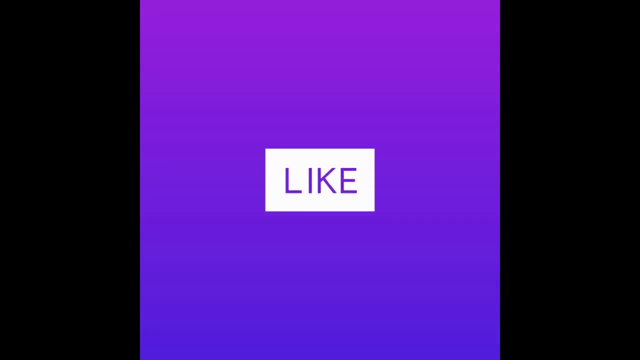 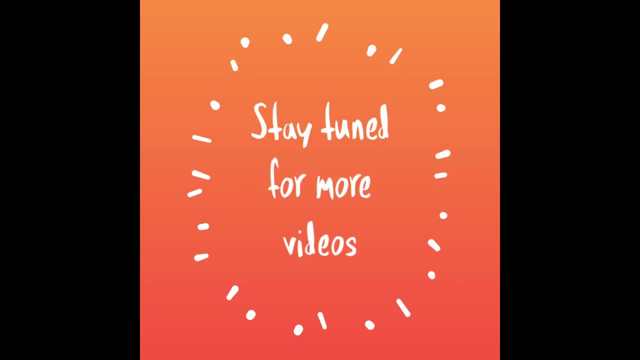 Thank you, Thanks for watching, Thank you.